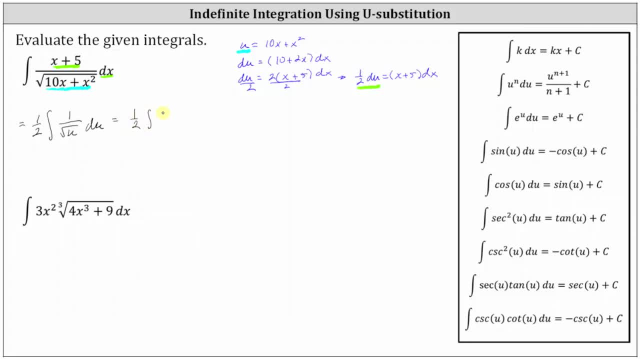 Let's rewrite this as: one half times the integral of one divided by u to the power of one half du. In order to apply the power rule of integration, we now need to write one divided by u to the power of one half as u to the power of negative one half. 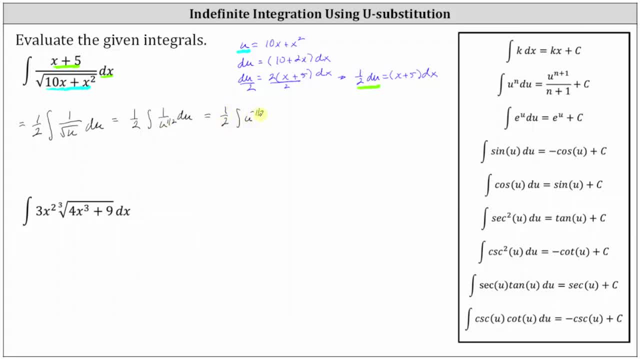 which gives us one half times the integral of u to the power of negative, one half du. And now we integrate with the spectra, spectra u, which gives us one half times u to the power of negative. one half plus one is positive one half divided by positive, one half plus c. 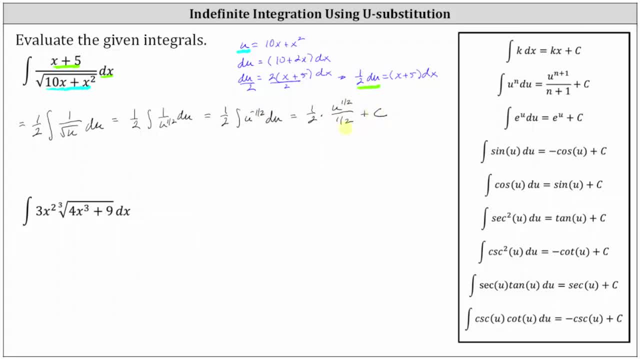 Simplifying further: dividing by one half is equivalent to multiplying by the reciprocal of two over one, which gives us one half times two over one times u to the power of one half plus c. Simplifying, we just have u to the one half plus c. 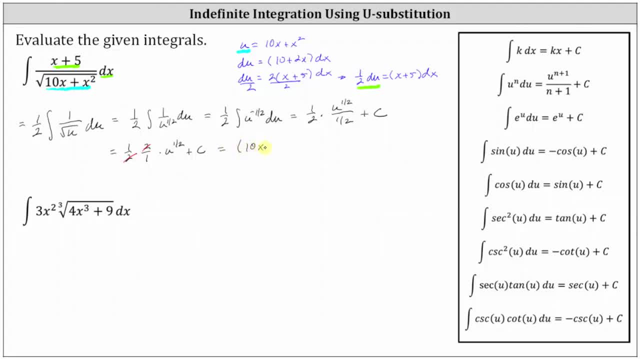 Which, in terms of x, is the quantity 10x plus x squared raised to the power of one half plus c. Or, if we want, we could write this as the square root of the quantity 10x plus x squared plus c. And we often use big F of x for the antiderivative. 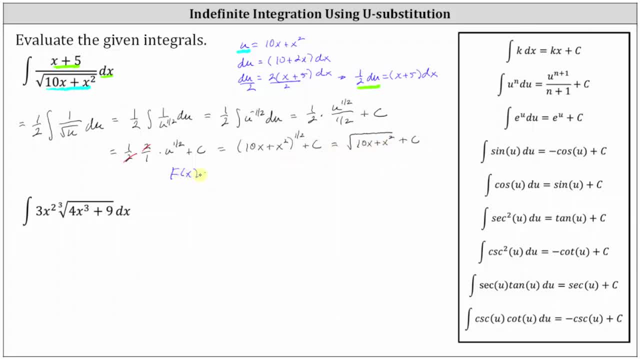 or indefinite integral. We can say: big F of x is equal to the square root of the quantity 10x plus x squared plus c. This is the family of functions. This is the family of functions whose derivative is equal to the given integrand function. 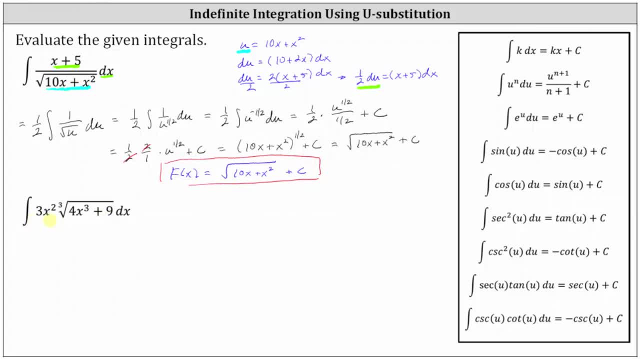 Looking at the next example, analyzing the integrand function, we have a degree two, monomial, outside the cube root and we have a degree three, polynomial, under the cube root. And since the derivative of a degree three polynomial is degree two, we will let u equal the radicand. 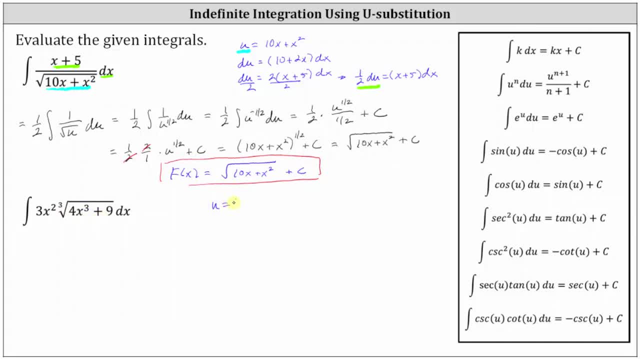 of four x cubed plus nine, Which means now: this is the cube root of u, which is equivalent to u, to the power of one third. And now we determine differential u, which is equal to the derivative of four x cubed plus nine. 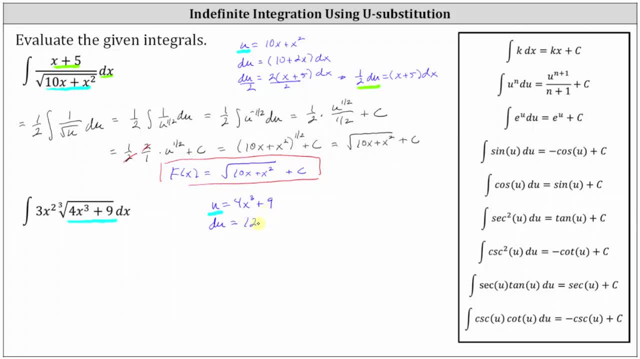 with respect to x times dx, which gives us 12x squared times dx. Notice, we have three x squared dx, not 12x squared dx. So we have an option here: We could divide both sides by four so that we have three x squared dx. on the right: or we can just solve for x squared dx. So we have an option here. We could divide both sides by four, so that we have three x squared dx on the right, or we can just solve for x squared dx. So we have an option here. We could divide both sides by four so that we have three x squared dx on the right, or we can just solve for x squared dx. 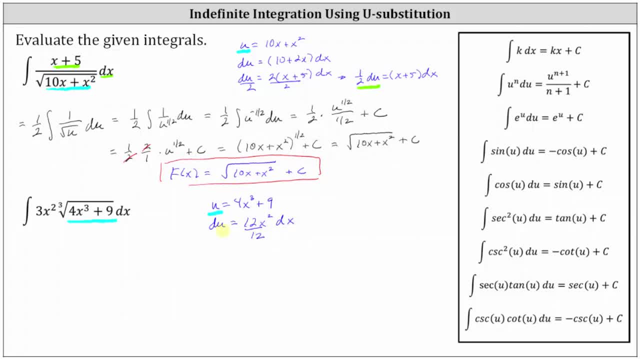 I'm going to go ahead and just solve for x squared dx, because it's not always easy to determine what to multiply or divide by for a perfect match. Simplifying now notice how we have: 1 12th du equals x squared dx. 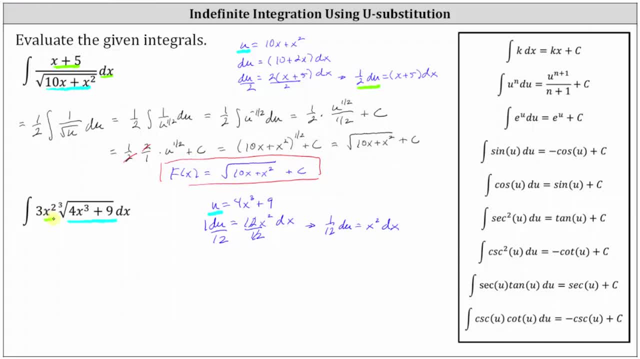 So, going back to the integral, we can factor out the three and now replace x squared dx with 1 12th du. So we're at the integral in terms of u. Again, we factor out the three, Then we have the integral of x squared dx is 1 12th du. 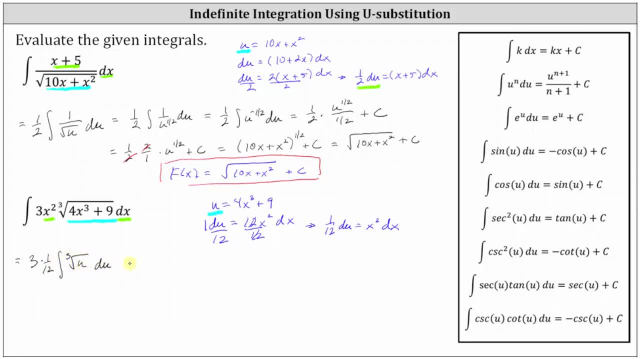 And then we have the cube root of u, which is equal to 3- 12ths, is 1, 4th times. the integral of the cube root of u is equal to u to the 1, 3rd du. And now we integrate with respect to u. 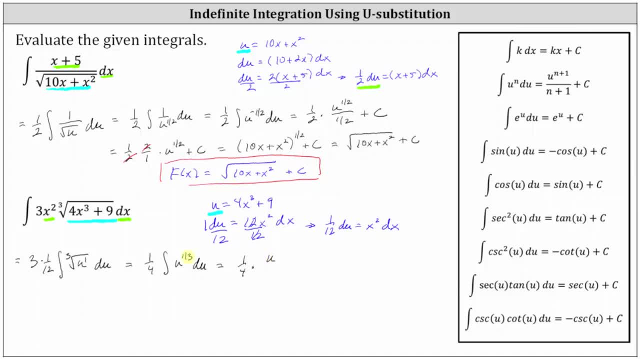 which is 1 4th times u to the power of 1 3rd plus 1, which is 4 3rds Divided by 4 3rds plus c. Dividing by 4 3rds is the equivalent to multiplying. 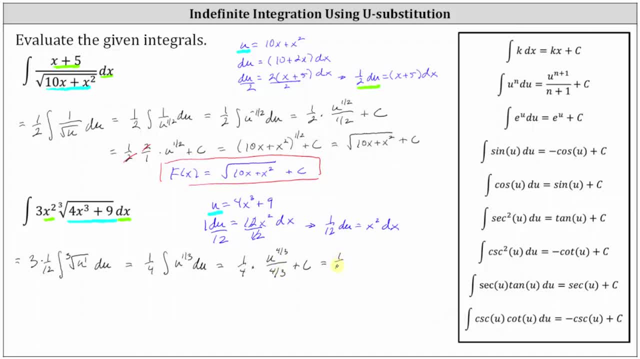 by the reciprocal of 3- 4ths, which gives us 1 4th times 3 4ths times u, to the power of 4 3rds, which, in terms of x, is the quantity 4x cubed plus 9. 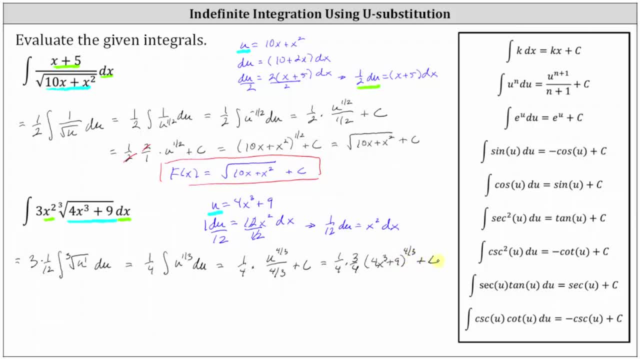 raised to the power of 4 3rds plus c. Simplifying one more time, we have 3- 16, times the quantity 4x cubed plus 9, raised to the power of 4 3rds plus c. 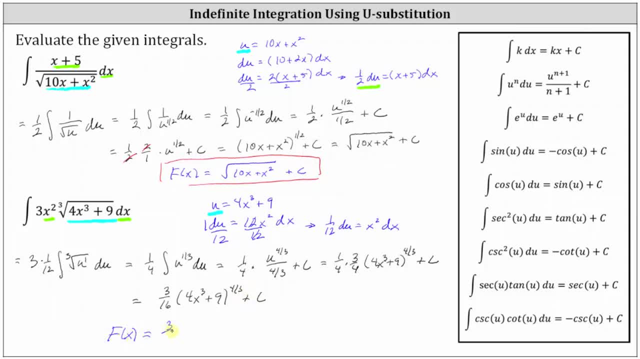 which can also be identified as big F of x, which once again, is the family of functions whose derivative is equal to the given integrand function. I hope you found this helpful.